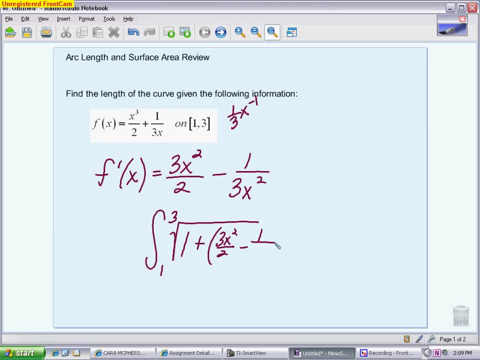 So 1 plus this, 3x squared over 2 minus 1 over 3x squared, That whole thing squared. So first thing is make sure, when you enter it in your calculator, you enter this denominator in parentheses, in its own parentheses. 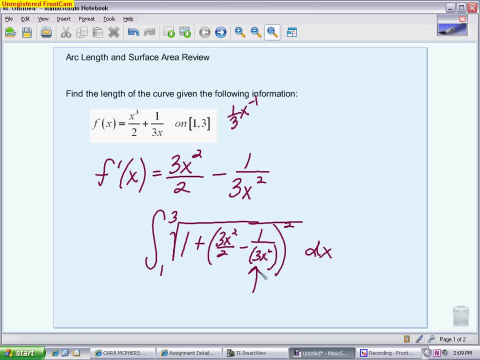 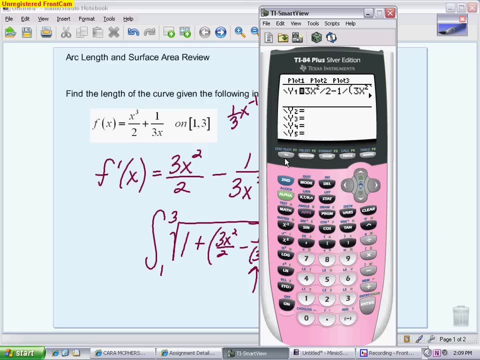 to keep it together. The other thing is it's probably going to be easier if you store that particular value in your calculator in y equals. So just to remind you how you do that, you're going to go into y equals and you're going to type in that function that you want to store as your y sub 1.. 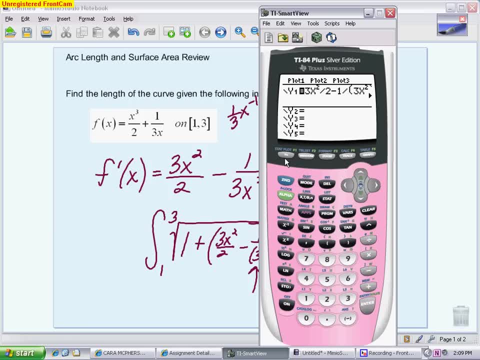 So you notice that I already did this. So I typed in 3x squared divided by 2, minus the 1 over the quantity 3x squared And then, just so you can see, it's all there. Kind of see that there. 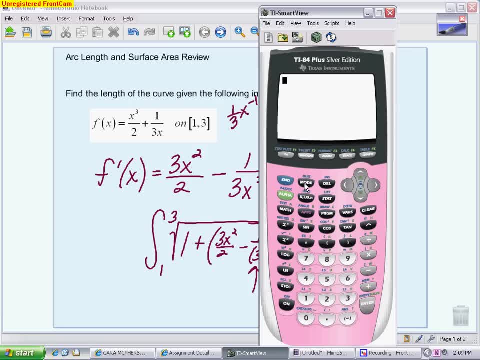 And then I'm going to quit out of that. And when I go to enter in my calculator, I'm going to go to math 9. Type in your boundaries 1 to 3. And then your square root of 1 plus. 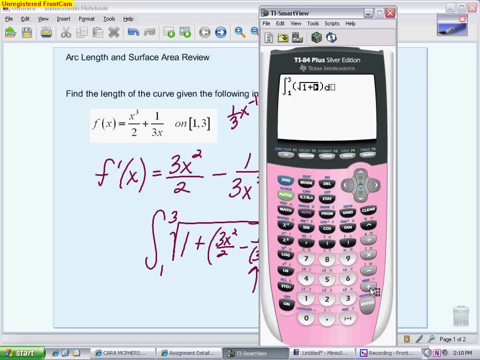 And now you want to get that y1 back. The process for doing that is you go to the variables button, or the one that looks like vars, Go over to y variables, Hit function And then, whatever you called it, we did it y1.. 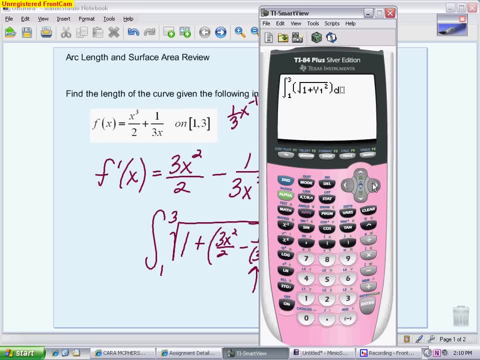 Don't forget to square it And then put your x here. Your answer: a lot of these are going to be decimals that will not become fractions. If you test, I'm pretty sure this is a decimal. Yeah, you're not going to get it to change. 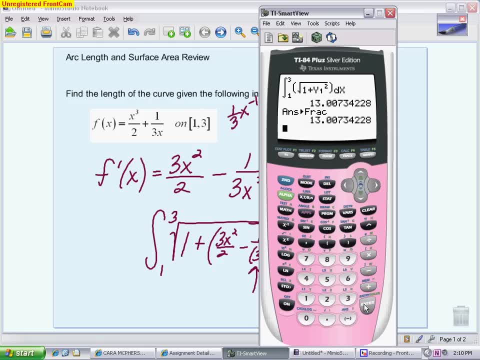 Just get in the habit of writing the three decimal places. Remember that if it wants a unit, it is just units. It is not anything that's being squared or cubed, because this is not area or volume, It is simply a length. 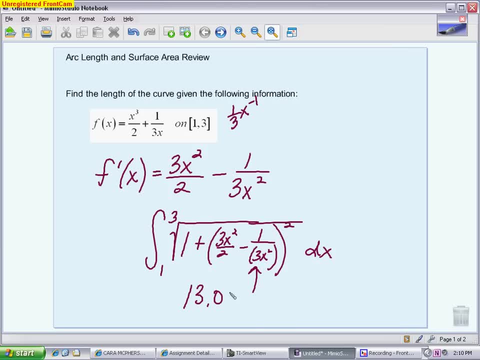 So your answer would be 13.007.. When I grade this on the test, I'm looking for three things. I'm looking for an accurate derivative, an accurate setup and then your final answer, correct to three decimal places, The other topic that we did, the second half of 7.4. 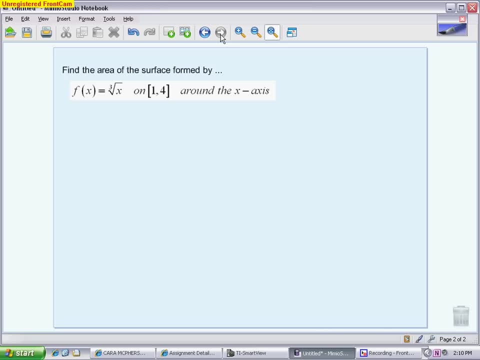 was finding surface area And I tried to use the same wording that you should expect in the test. It will usually say: find the area of the surface form by, And then it will give you three things: The function, the interval, and those are always an x interval. 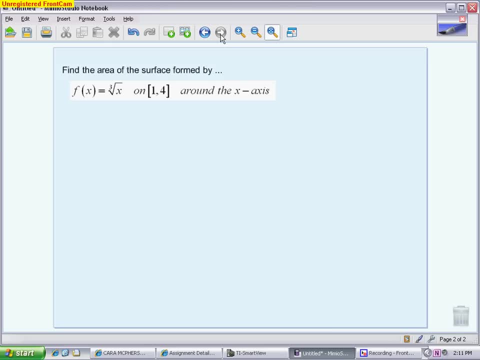 and then what we are revolving. And that's the one piece that's going to make the formula a little different. First thing you want to do, as you did with arc length, is find the derivative. So, remember, think of this as x to the 1 third. 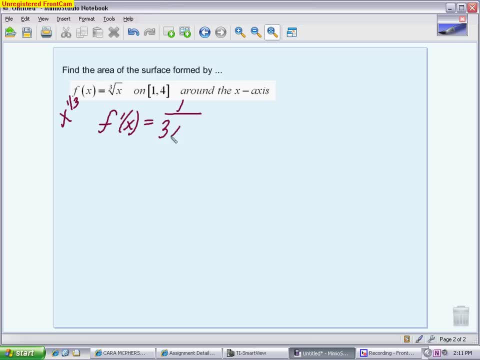 So you're going to do power out front, power 1 less. You're going to end up with 1 over 3x to the 2 thirds. Your formula has a 2 pi out front integral from 1 to 4.. 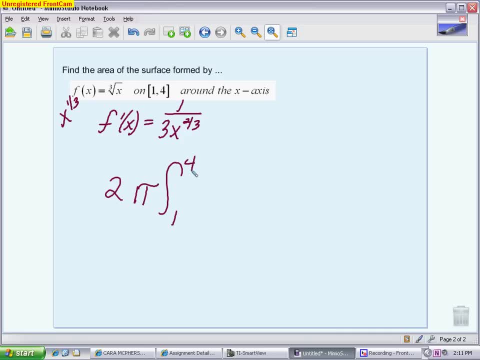 The one thing that's different about surface area is you have to put your original function if you're going around the x-axis and your x if you're going around the y-axis. So we're going to put our original function around it. 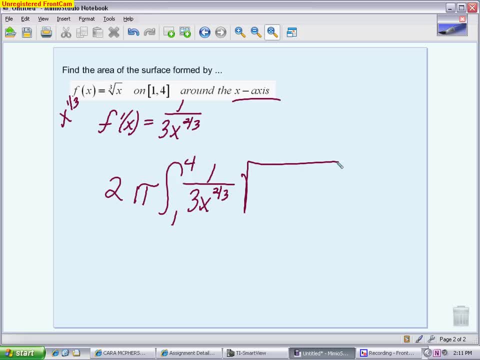 because we're going around the x-axis And then we're going to take the square root of 1 plus that squared, So I'm going to square it out. When I square it out, I get 1 over 9x to the 4 thirds. 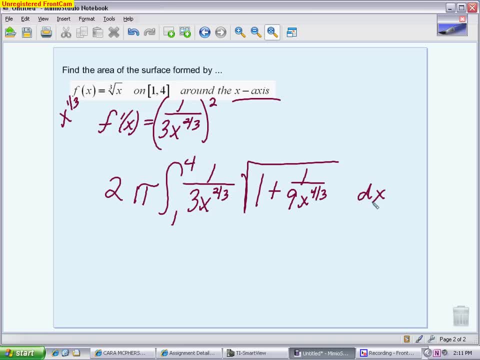 So here's my setup. Again, same point system. I'm looking. did you take your derivative correctly? Did you set it up correctly? And then that last point is putting in your calculator, because sometimes that's where you might lose a point. 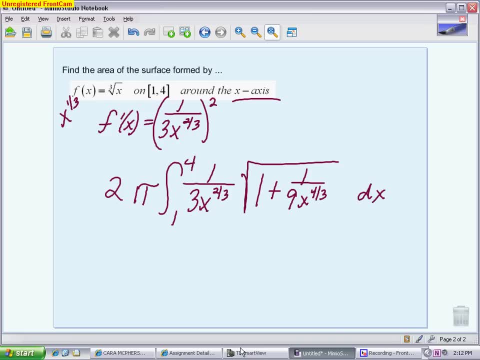 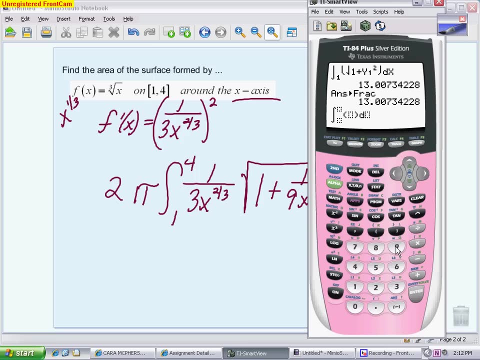 It just can be 1 parentheses, 1 sign can kind of throw it off. When I do this in here, I'm not going to store anything as y1.. It's not really as complicated. I am going to just go straight to your integral function. 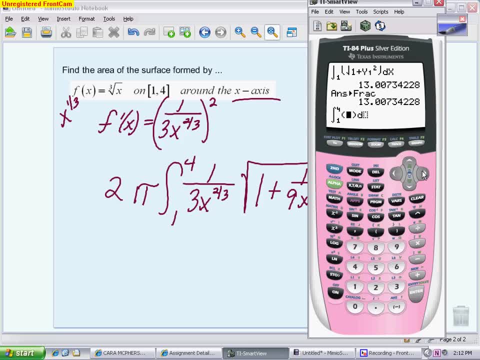 going from 1 to 4.. Put in your original function And here's again where you need parentheses: 1 divided by parentheses, 3x to the 2 thirds. Older calculator will also need parentheses around that 2 thirds or using the alpha button to make it a fraction. 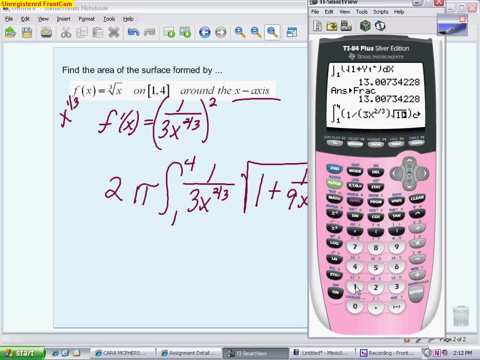 And then square root of 1 plus your 1 divided by and again, I need parentheses around this denominator: 9x to the 4 thirds. Get out of the parentheses, Get out of the square root. There's your answer. 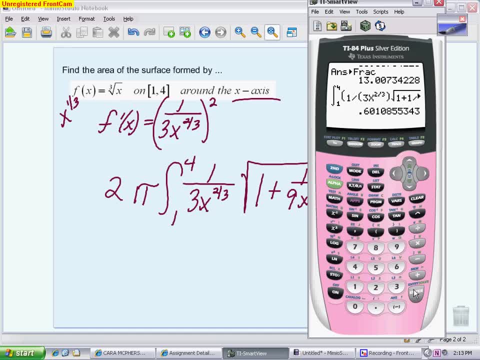 And again, you want to make sure that you double it. So you're going to double it, So times 2.. And finally, put a pi in there, And I don't think this one's going to work out to be a fraction either. 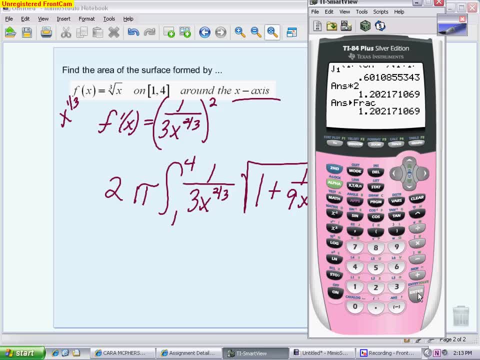 So again, hopefully everything that's what you're looking for, Everything's set up correctly. You can double check Where am I going? I'm going to go back and I'm just going to look at the way I entered, just to kind of review all that with you. 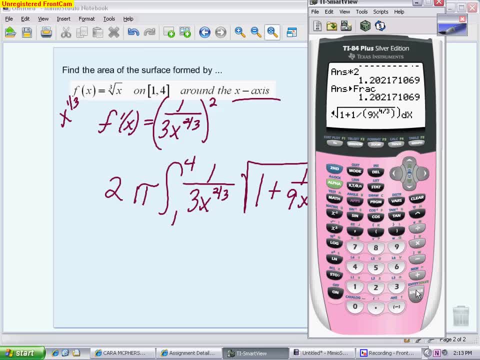 just to make sure everything was entered correctly, Because that's definitely where the bigger questions seem to come from. So again we have the original function in front of the radical, because we're revolving around the x-axis. If you were revolving around the y-axis, 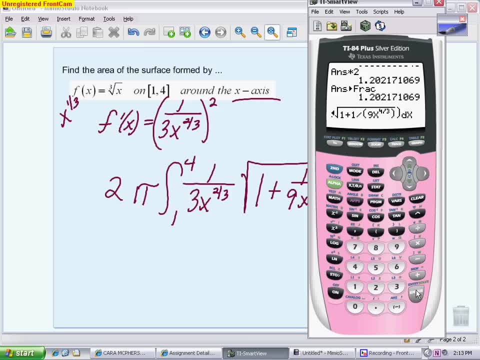 you would just put an x there. We have 1 plus the derivative squared, So you can either square it out by hand or you can leave it in parentheses and then put a squared there. We get that answer and we multiply it by 2,. 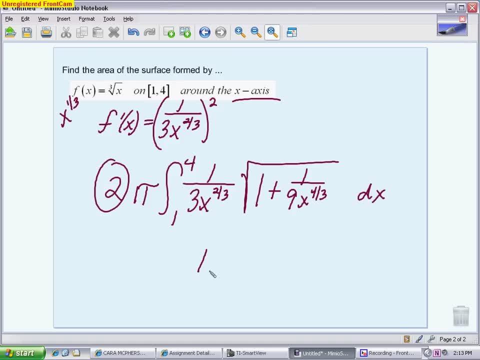 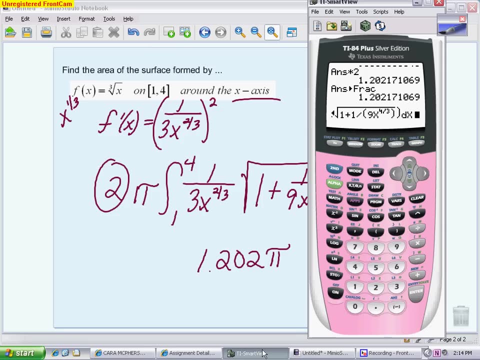 because of the 2 that's in front of here, And then we're going to write our answer, three decimal places, and include pi. If you want to multiply pi through, you can. If you want to just leave it, Because the 1.202 pi, it's a little more concise. 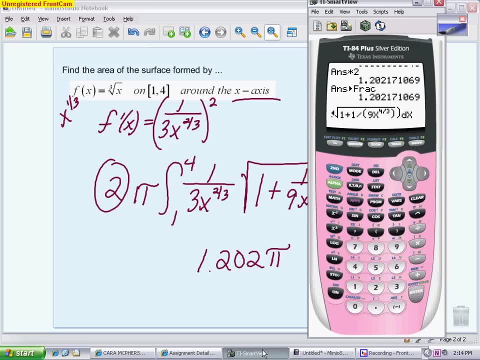 a little less rounding to worry about. And that's how you do. surface area Units would be units squared. Again. I'm not going to get real picky with asking for unit, But because it is an area unit, it's a surface area. 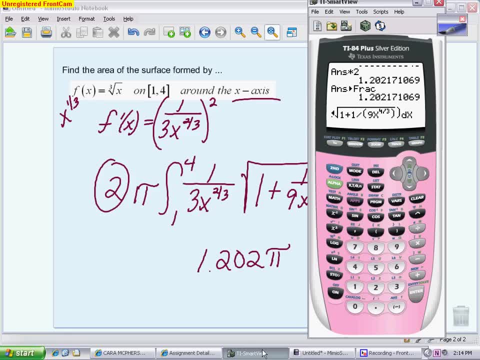 it would be units squared. So this just takes you through basic application. You should be able to set up and use your calculator to integrate any arc length and any surface area problem that you're presented with. 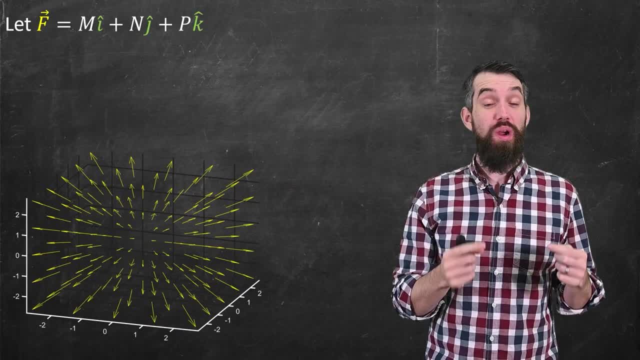 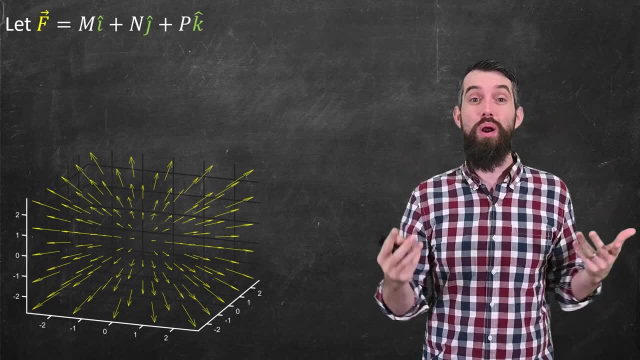 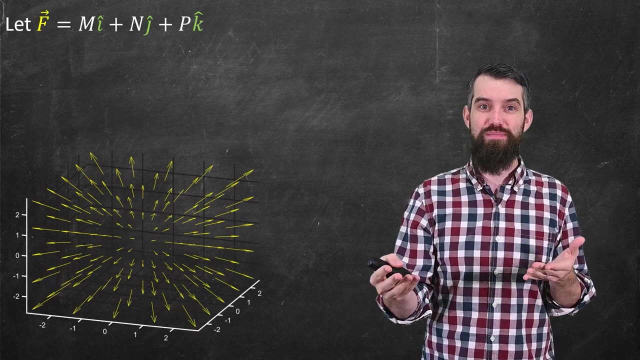 In this video we're going to see the final major theorem of our vector calculus course, the divergence theorem. So what are we talking about? I'm going to begin with the vector field. This is a three-dimensional vector field. It's got components m, n and p And the vector field. 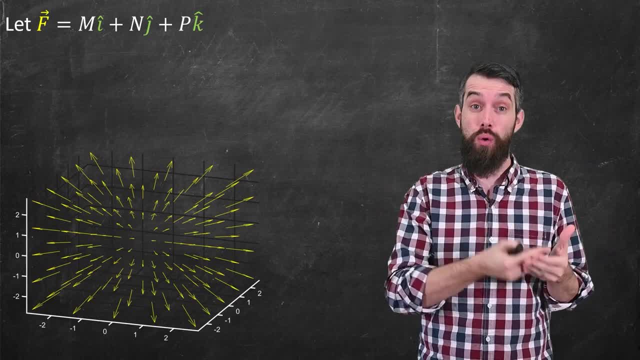 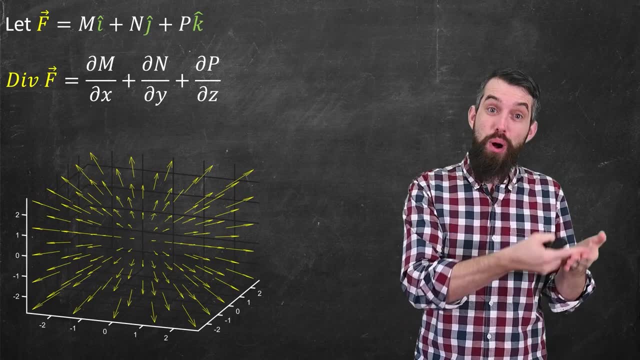 I've given is a source vector field. Everything seems to be exploding out from the origin. Then the divergence is defined to be the sum of the partial derivative of the first component, n with respect to x, the second, n with respect to y and p with respect to z. 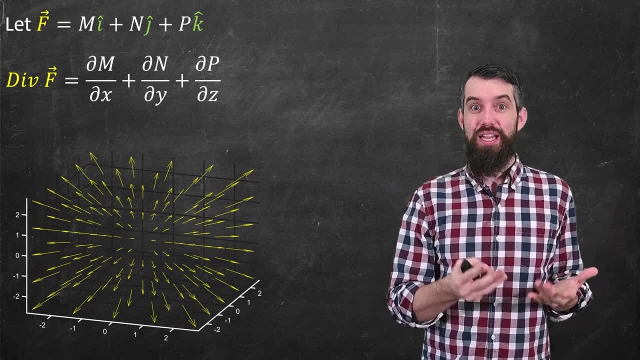 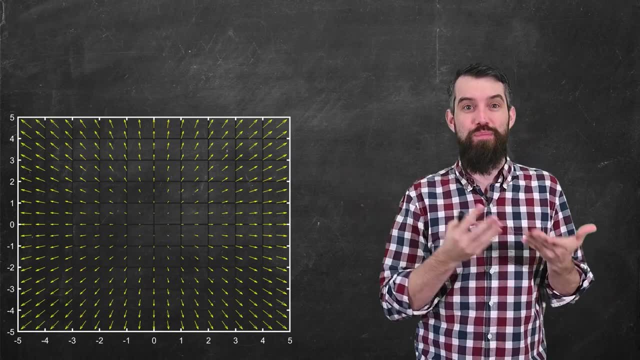 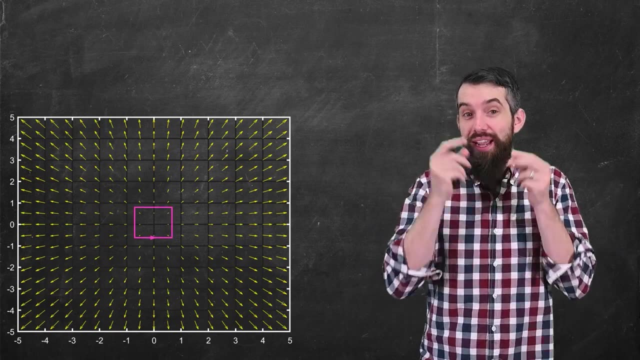 That gives the divergence, Okay, but what is this Now? we've actually seen divergence before in the two-dimensional case. So there we were talking about the same basic type of field, a source field, but in two dimensions, And what we studied was the effect on a tiny little.